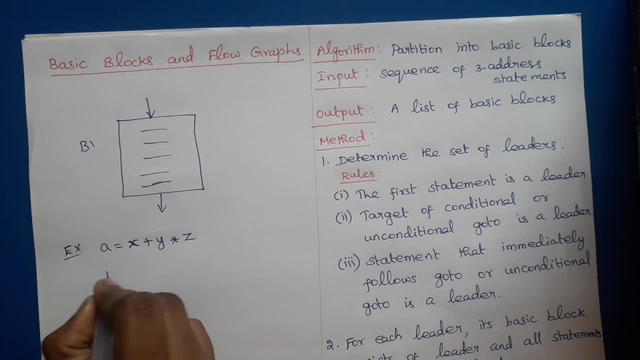 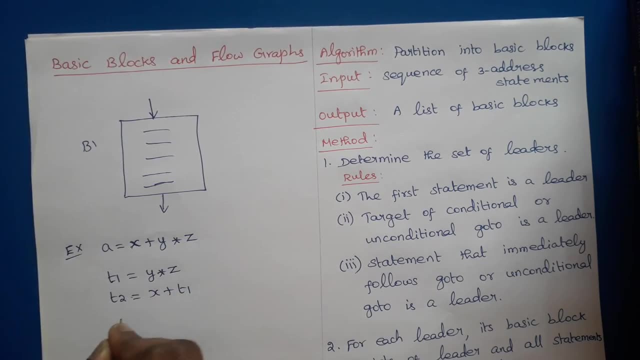 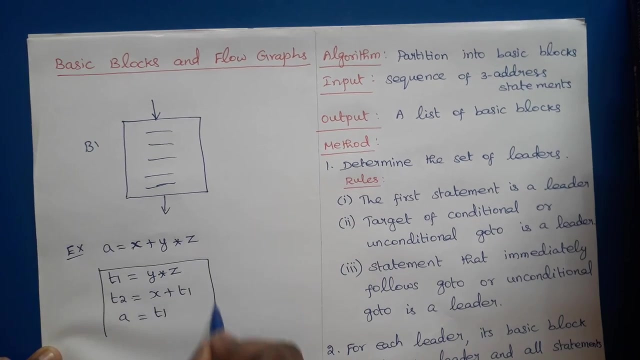 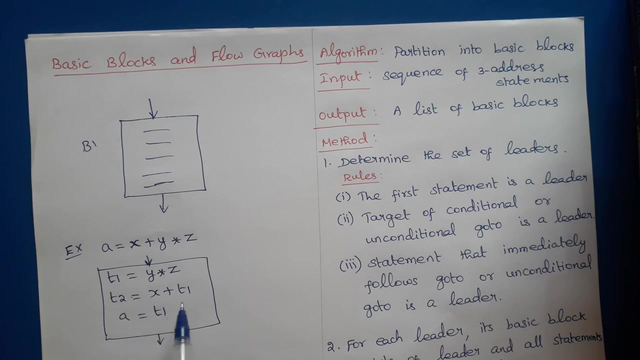 three address statements for this example is: T1 is equal to Y star Z, T2 is X plus T1, and A equals T1.. So this sequence, that is, these three statements, can be in a single basic block. So here flow of control enters at the beginning and leaves at the end, and there is no branching. 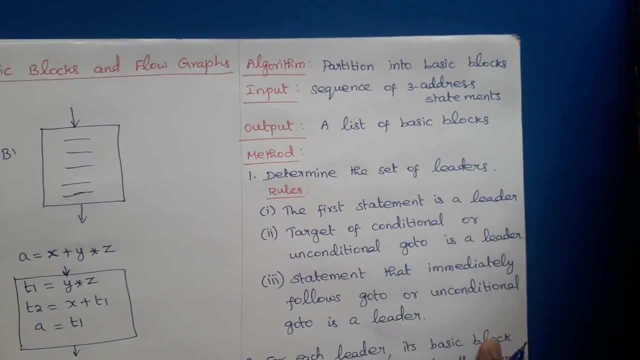 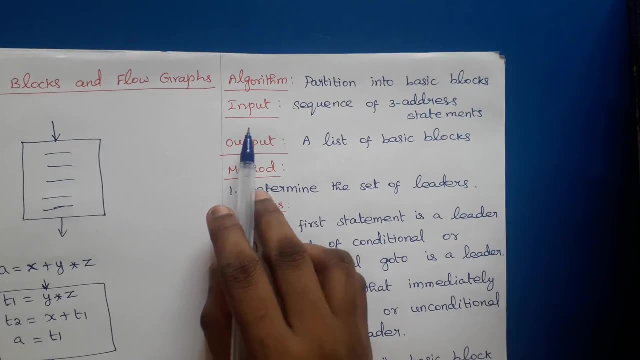 statement in the middle of the statement. So this is an example. Now we have to see about algorithm for partitioning the three address statements into basic block. So here the input is a sequence of three address statements. So from the three address statements only we are going to 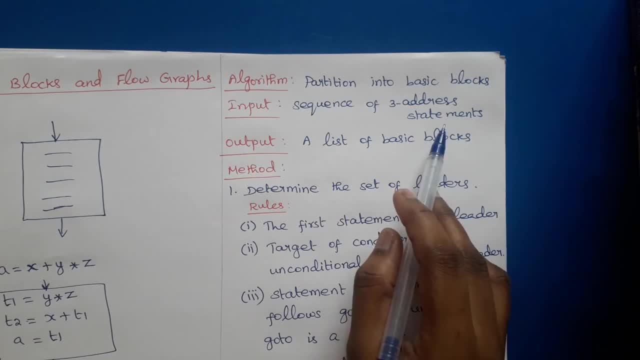 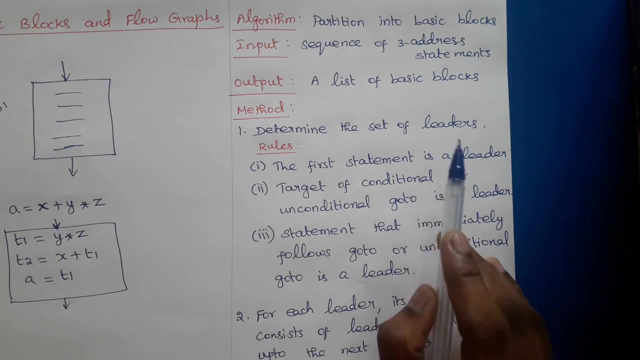 construct the list of basic blocks. So input is sequence of three address statements, Output is a list of basic blocks method. So here there are two steps. First we need to find the set of leaders. Leaders means it's a first statement in a basic block. So in this basic block leader is T1 equals. 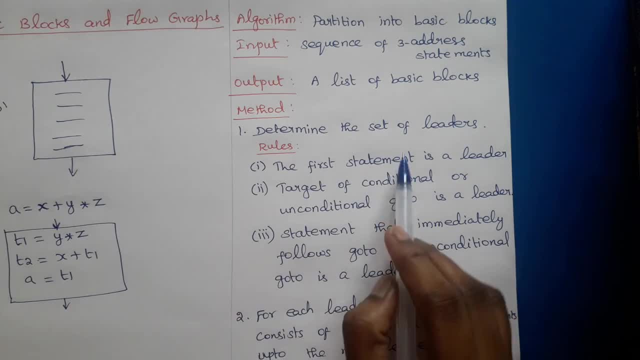 Y star Z. So first statement in a basic block is called as leader. So first we need to find the set of leaders for the basic block. So there are three rules for finding the leaders. First rule is the first statement is a leader. 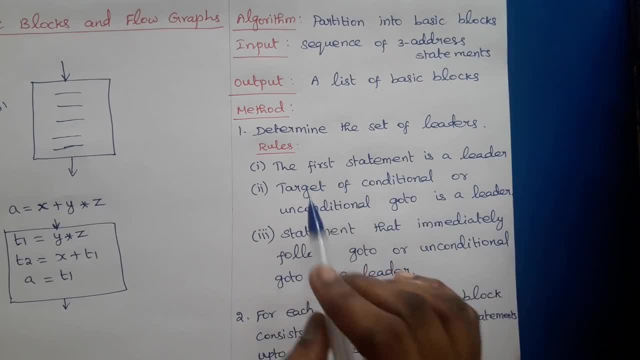 First statement of the program in the sequence of three address statements given means the first statement is a leader. This is first step. Second rule is any statement that is a target of conditional or unconditional goto is a leader. So, for example, goto 3 is given means that 3, the 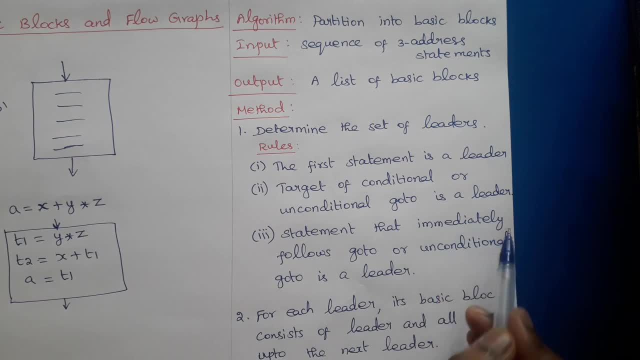 Target of unconditional go-to or conditional go-to is a leader. So this is the second rule. Third rule is any statement that immediately follows conditional or unconditional go-to is a leader. So these are the three rules. First statement is a leader. Target of conditional or unconditional go-to is a leader. 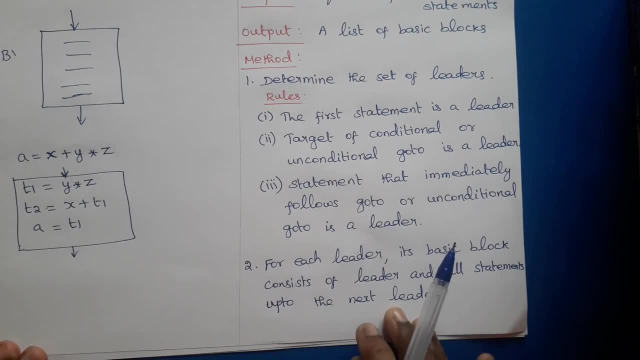 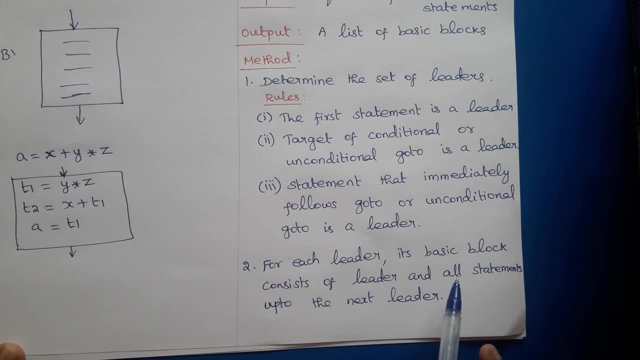 Statement. immediately follows: go-to, or unconditional go-to, is a leader. So, after finding the leaders, for each leader we have to build one basic block. So that basic block consists of leader statement, leader and all statements up to, but not including, the next leader. 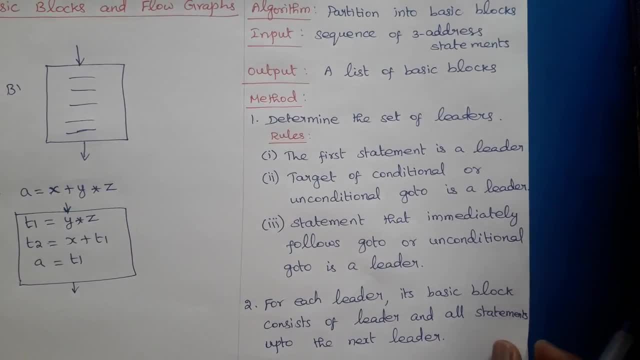 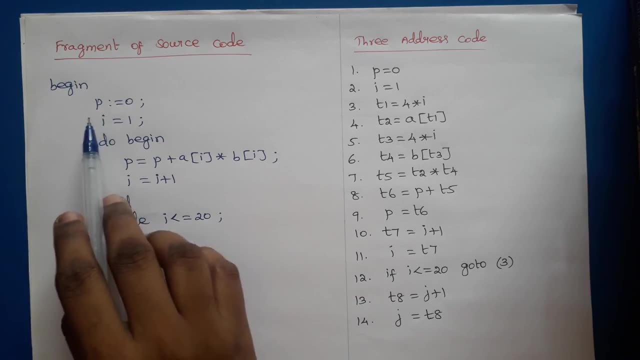 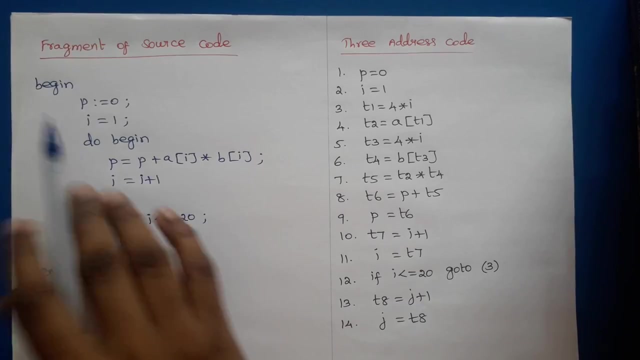 So this is the second rule for constructing the basic blocks. So consider an example fragment of source code. So this is the fragment of source code given and this is the corresponding three address code generated by the intermediate code generator, And assume that this is a given source code. 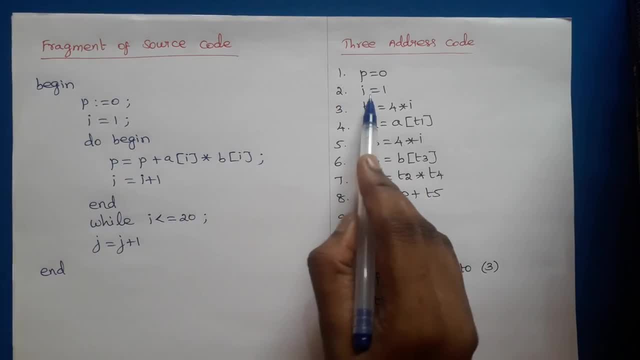 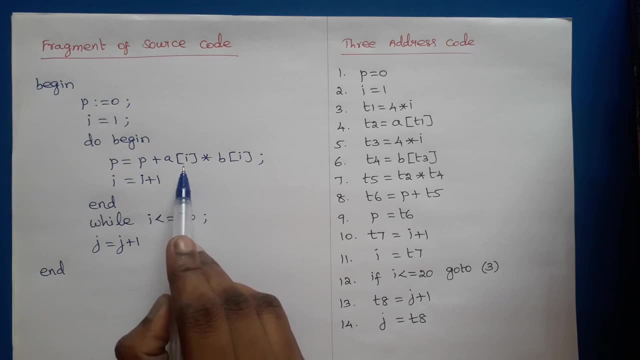 So first three address statement is P: P equals 0, then I equals 1, and this is a loop. Do I loop is given, So first we need to calculate this. So assume that here I, this index occupies 4 bytes. 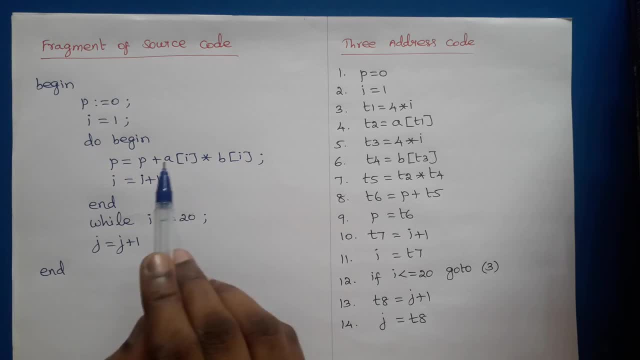 So if A of 0 is stored in 101, then A of 1 must be in 104, right, Each integer occupies 4 bytes, So first we have to calculate this index. So T1 is equal to 4 star I. 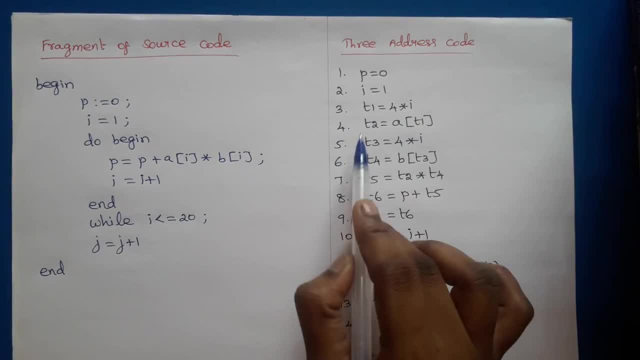 4 should be multiplied. So 4 is multiplied with I everywhere. Then T2 is equal to A of T1.. Similarly, T3 equals A of T. sorry, 4 star I. Then T4 is equal to T4 is equal to B of this T3.. 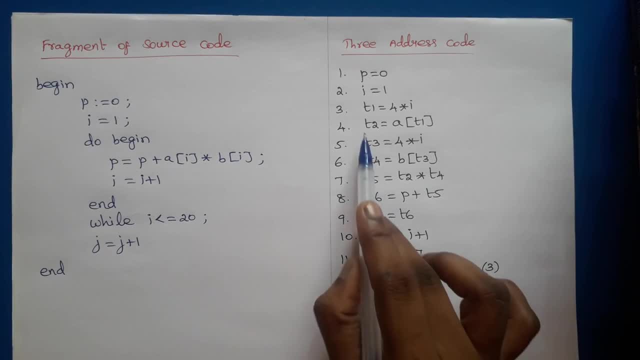 Then this multiplication should be performed, So T5 is equal to T2, star T4.. T2 consists of A, of T1 and T4 is B. So this multiplication, Then T6 is P plus T5, P plus T5.. 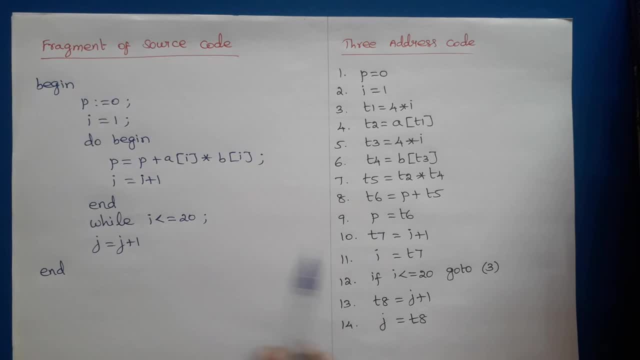 Then this P is equal to T6.. T6 must be assigned to P. Then I equal to I plus 1 should be calculated. So temporary variable 7 is equal to I plus 1.. Then this T7 is assigned to I. 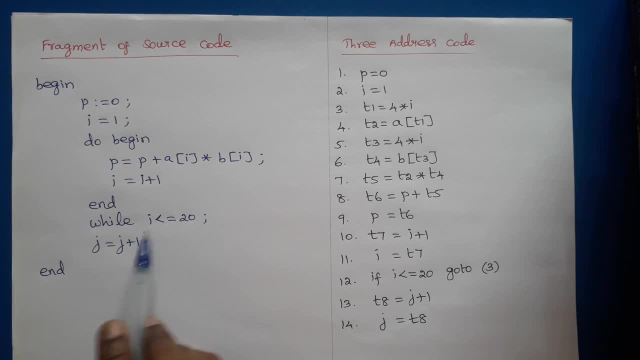 Then conditional statement is coming here. So if I less than or equal to 20 go to, this is a loop. So if this condition is satisfied, again we need to perform this set of statements. So if this condition is satisfied, again we need to perform this set of statements. 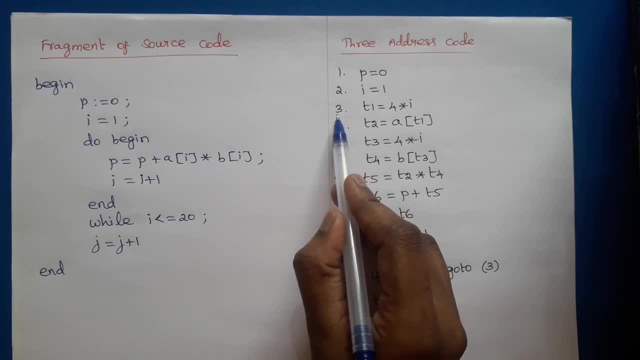 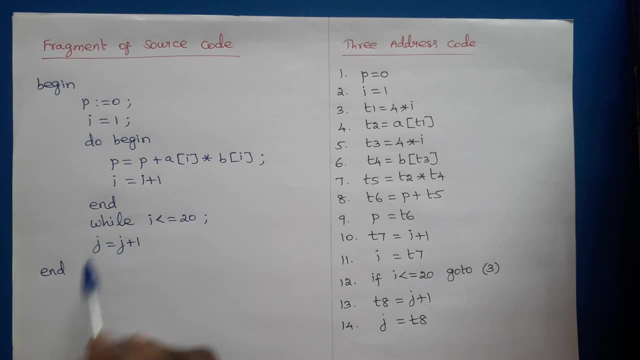 Execute this set of statements. So it starts with the number 3.. Statement number 3.. So if I is less than or equal to 3, go to 3.. Then after this, J equal to J plus 1 is there. 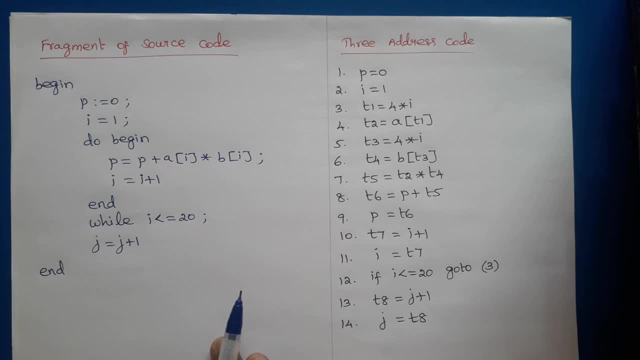 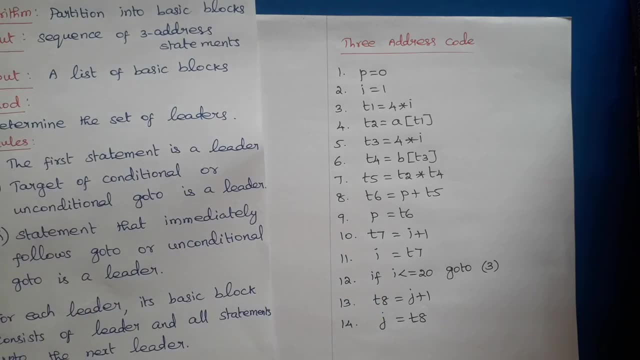 So T8 is equal to J plus 1. J is equal to T8.. So now from this 3 address statement we are going to construct the set of basic blocks. So what is the algorithm? First we have to find the leaders. 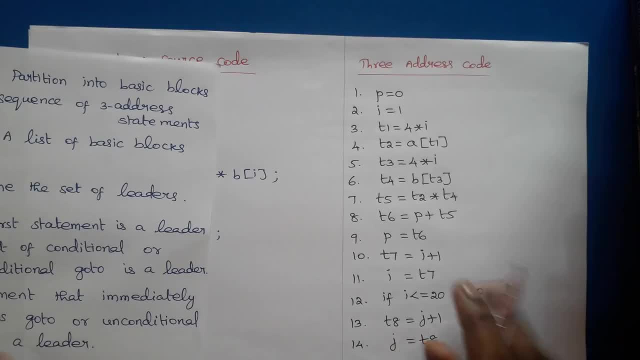 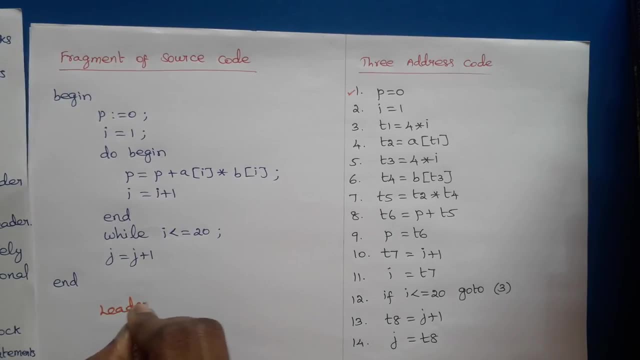 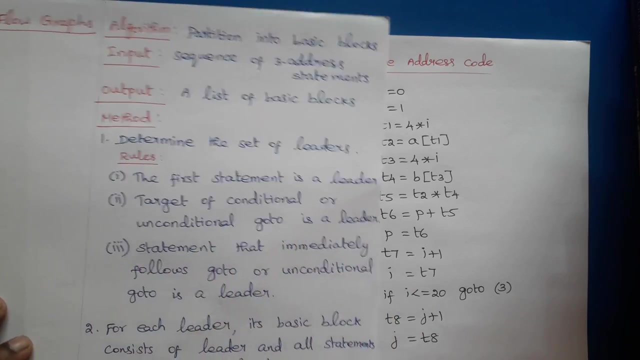 So what is the rule for Leader? First statement is a leader. So first statement is a leader. So statement number 1 is a leader. So set of leaders are 1.. Then target of conditional or unconditional go to is a leader. 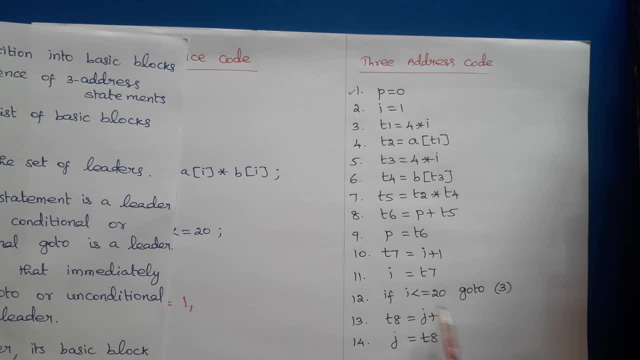 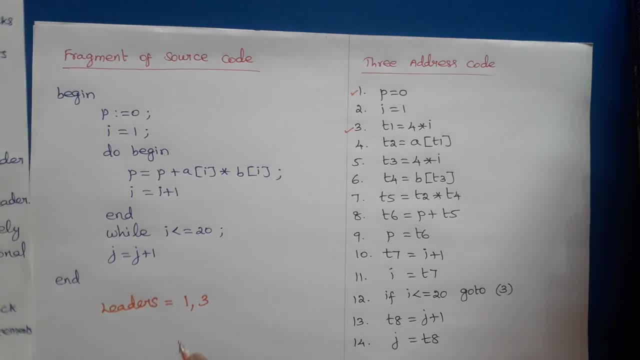 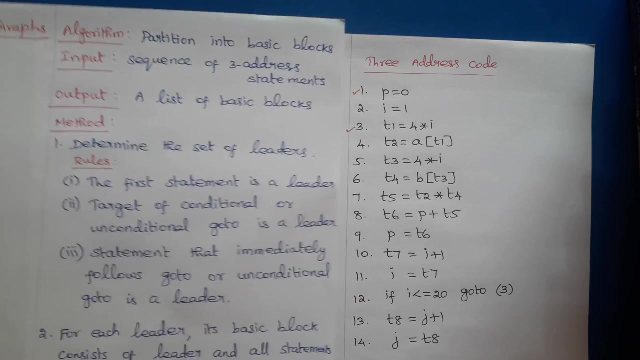 So here there is a conditional go to. So what is the target of this conditional? go to 3.. So statement number 3 is a leader, 3 is a leader. Then, as per Third rule, any statement that immediately follows go to or unconditional go to is a leader. 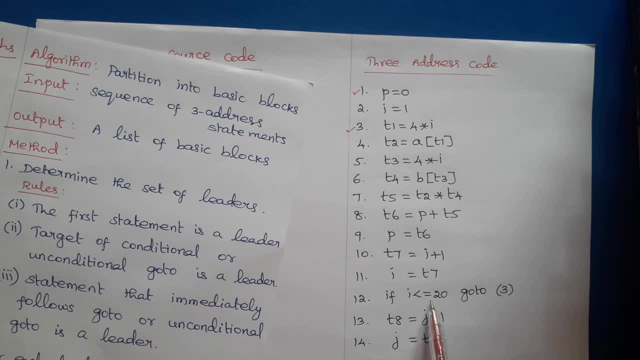 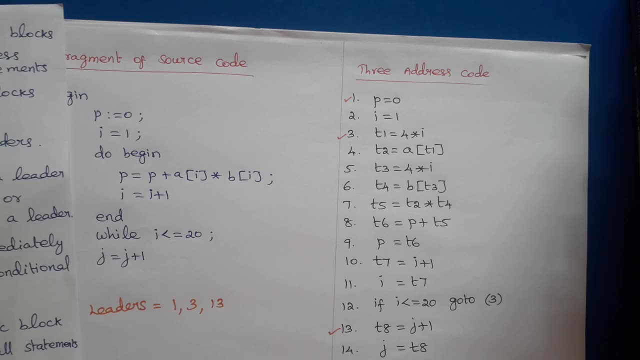 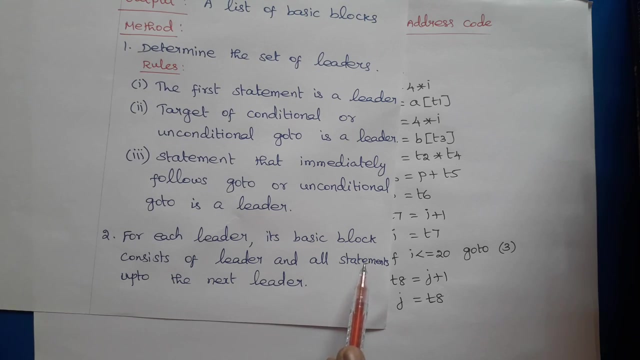 So here, conditional go to- is there Statement that immediately follows this conditional go to means 13.. So 13 is a leader. Now we have to construct a basic block for each leader. So for each leader we have to construct a basic block. 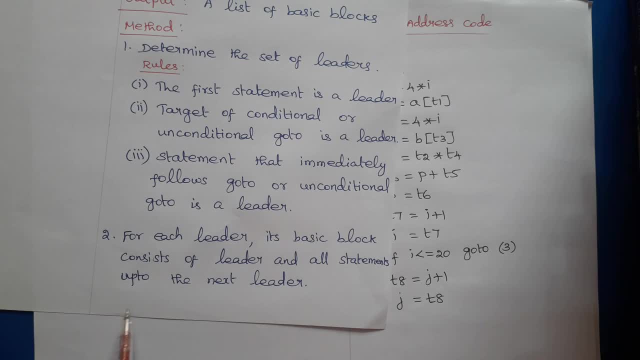 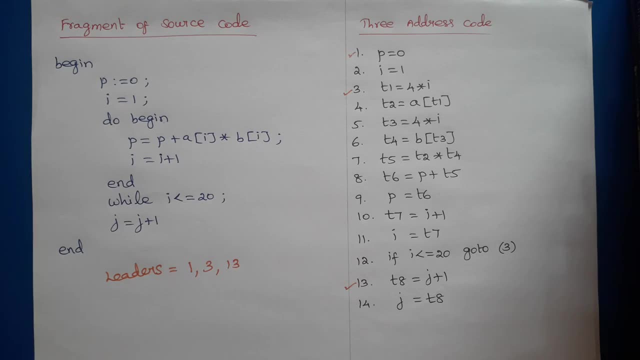 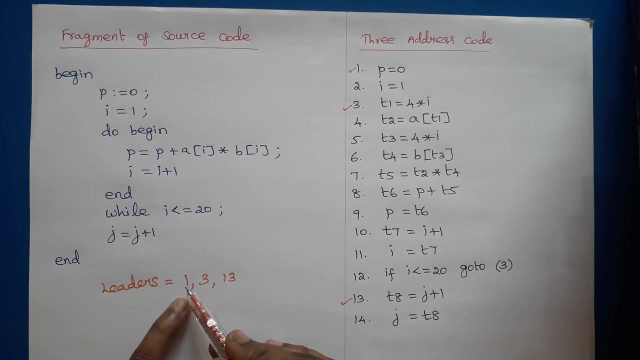 That block consists of leader and all statements up to but not including The next leader. So there are three leaders. So we will get three basic blocks for this three address statement. First basic block consists of statement number 1 and 2.. Statement number 1 and 2.. 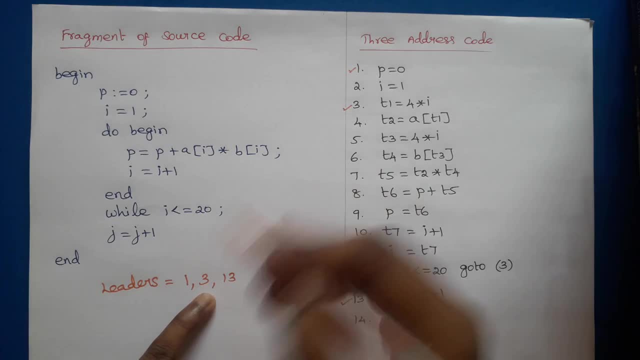 We should not include statement number 3 because it says another leader. So this is one basic block, Then another basic blocks starts with 3 and ends with 12.. Right, Because 13 is a leader. It's a bunch, Right. 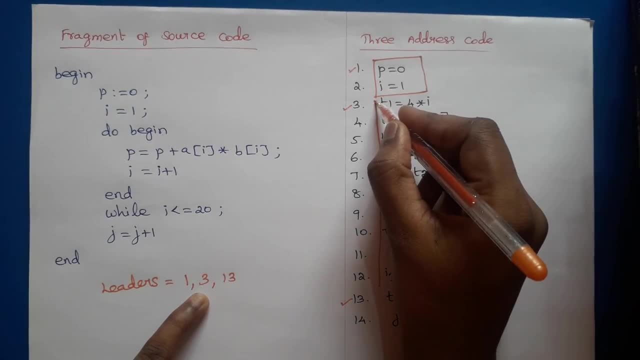 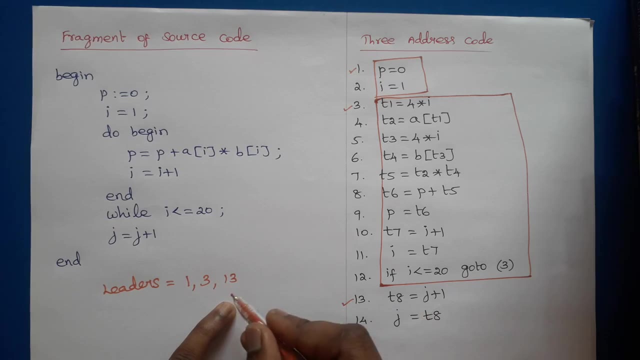 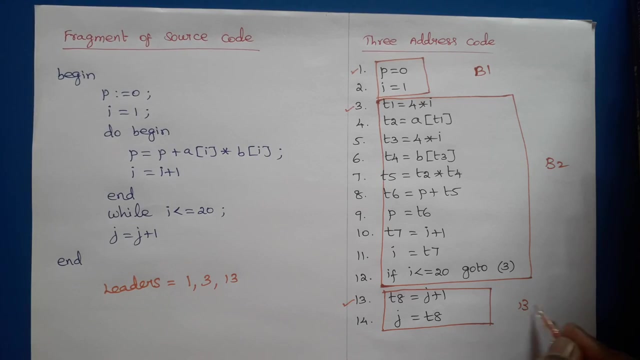 leader. so 3 to 12 is a basic block, then 13 from 13 to another leader. here 14 is the end of the statement. so these two statements form a third basic block. so here we have got basic block 1, 2 and 3. there are three basic blocks. now we will. 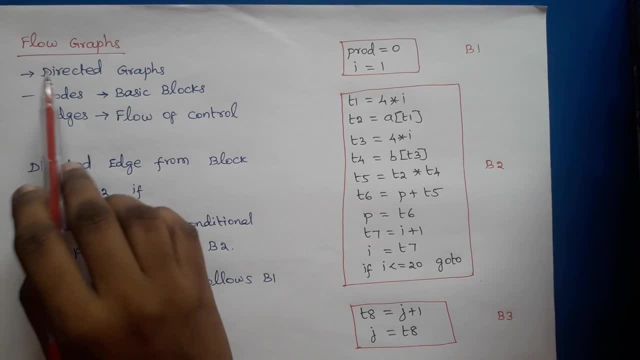 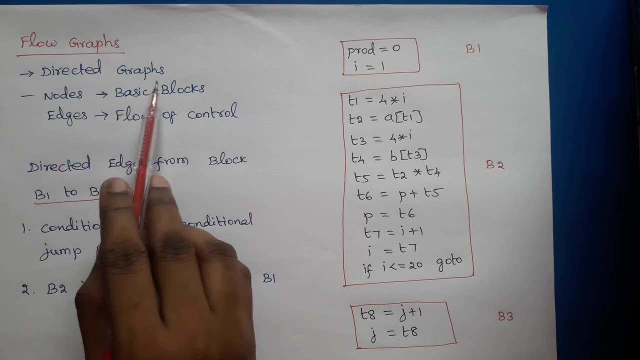 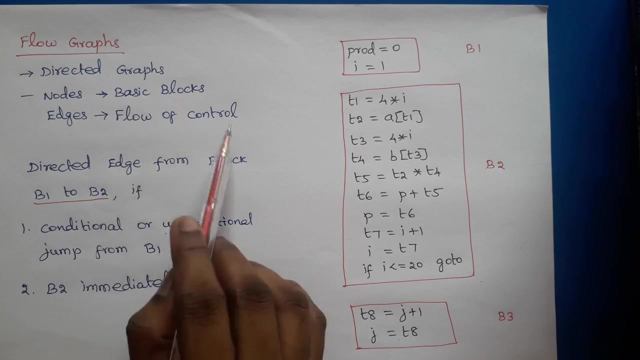 discuss about flow graph. so now we can add the flow of control information to the basic blocks by constructing the directed graph. flow graph is a directed graph in which nodes represent basic blocks and edges represent flow of control. that flow of control means the directed edges by means of directed edge. 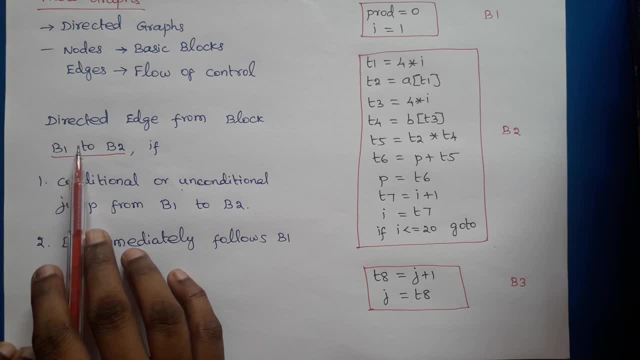 we can represent the flow of control, so we can draw a directed edge from block B1 to B2. if there are two controls, if there is a conditional or unconditional jump from B1 to B2, from block B1 to block B2, if there is a conditional or unconditional jump, then we 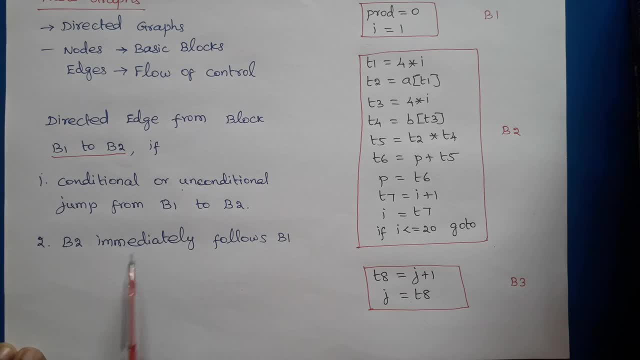 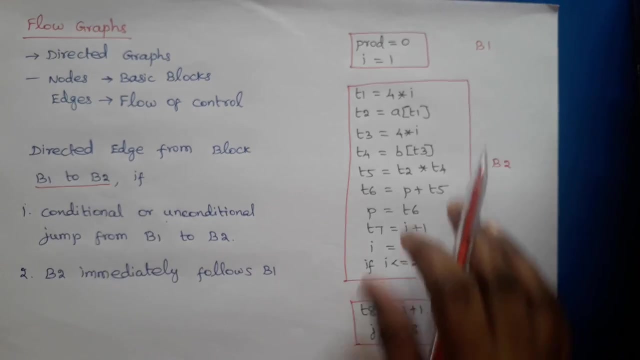 can draw an edge from B1 to B2. second step is if the block B2 immediately follows B1 in the program order, if B2 immediately follows B1, then we can draw an edge from B1 to B2. so there are two cases. so here consider this example here: 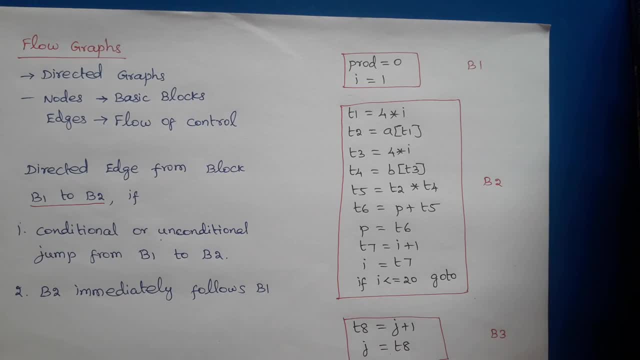 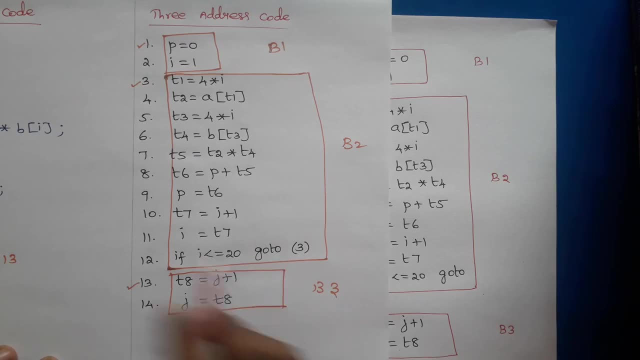 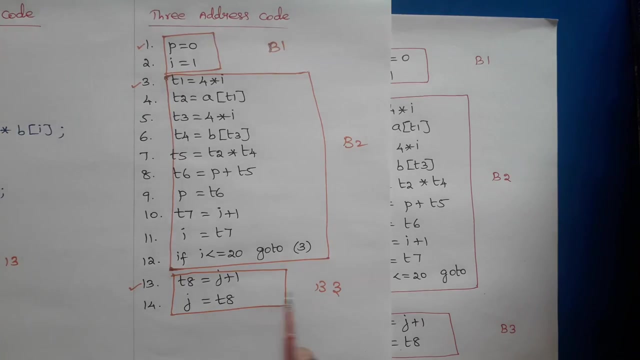 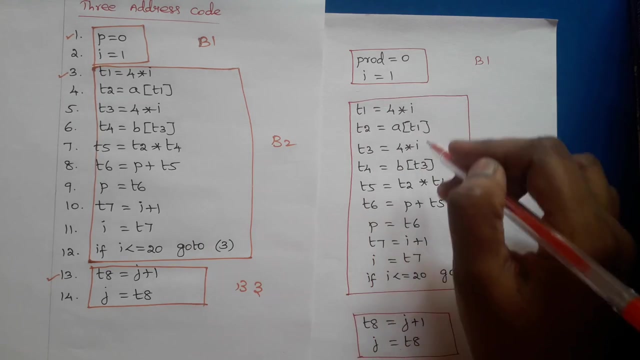 in the previous. actually here we have drawn the constructed basic block can go to three is used. three means it goes to three, the statement, right. the control will go to this statement. but here we don't write any number. so go to B2, the same statement. the control should go to the same statement. so instead of three, here we need to write. 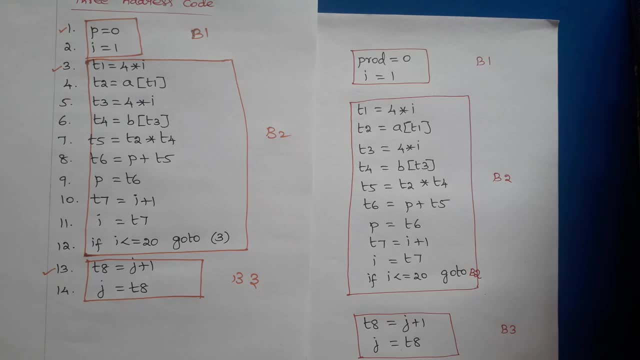 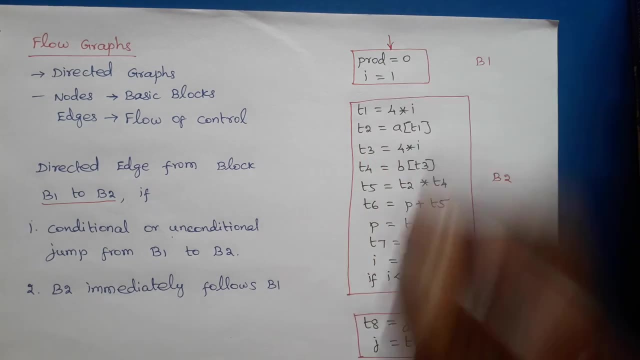 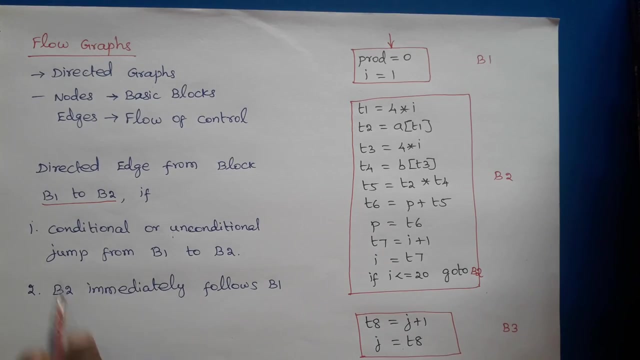 B2.. B2 should be written over here. So if the first, we will draw the diagrams, draw the edges based on the second step. So if B2 immediately follows B1, we can draw an edge. So in the program order, 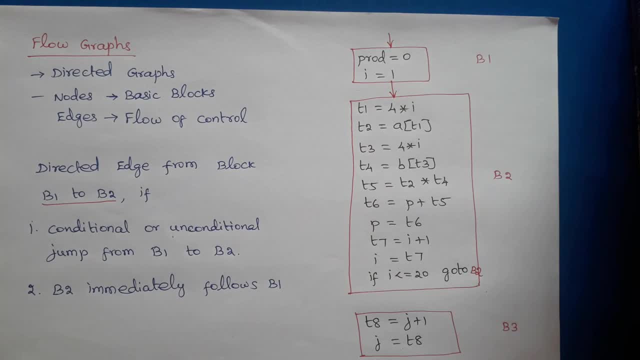 B2 follows B1. So we can draw an edge from B1 to B2.. Similarly, B2 can be followed by B1. Sorry. similarly, B2 is followed by B3. So there is an edge from B2 to B3 and we have to keep. 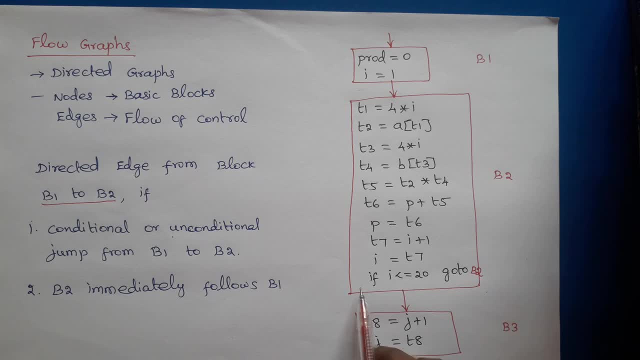 another point in mind, that here conditional goto is there. So if the block is having conditional goto in the last statement then we can draw an edge from that block to another block in the order. but if unconditional goto is there then this edge should not come over here. that first step alone.